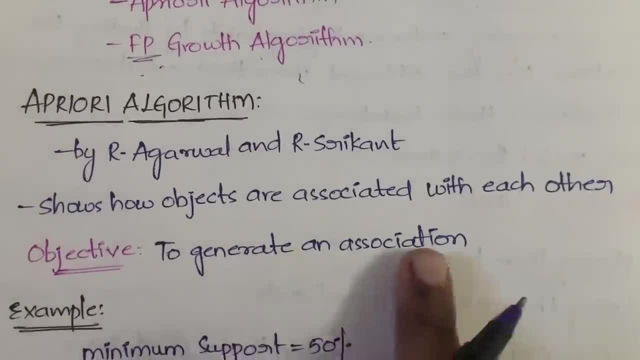 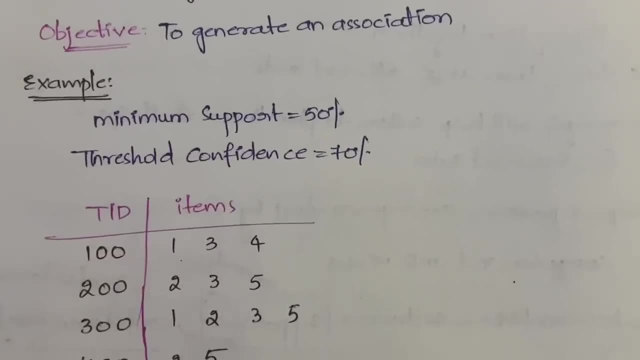 That's all Okay. for example, and our objective is to generate an association in this priori algorithm. Okay, don't worry With example, you will understand it. So, for example, first, before starting, we have to take the minimum support and minimum confidence. 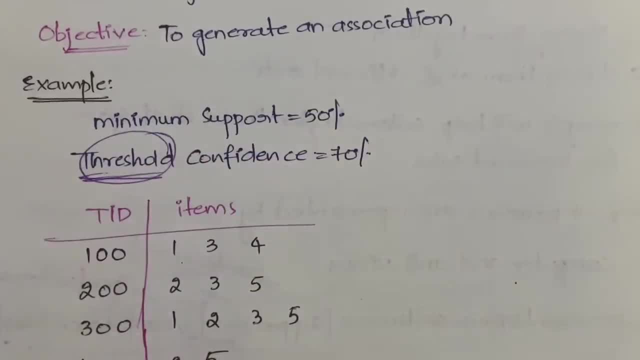 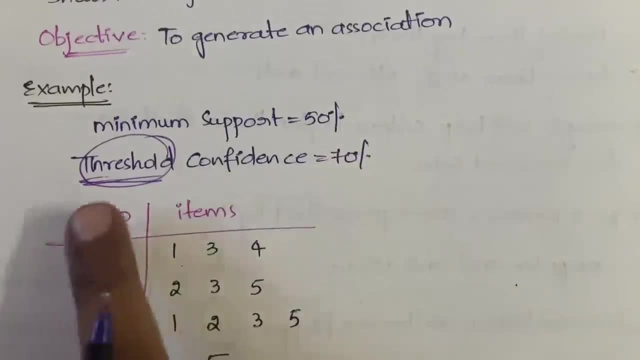 Threshold is nothing but minimum support or threshold support, minimum confidence, threshold confidence. anything you can say, Okay, you have to take the. we have taken minimum support as 50% and the threshold confidence as 70%. Okay, done Next. this is our example. 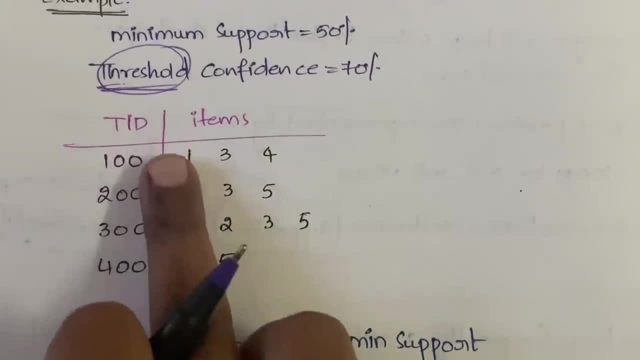 TID and items. TID is nothing but the transaction ID. For transaction ID 100,. we are having items like 1, 3,, 4. For 200, 2, 3,, 5.. For 300, 1, 2, 3,, 5. For 400, 2,, 3, 5.. 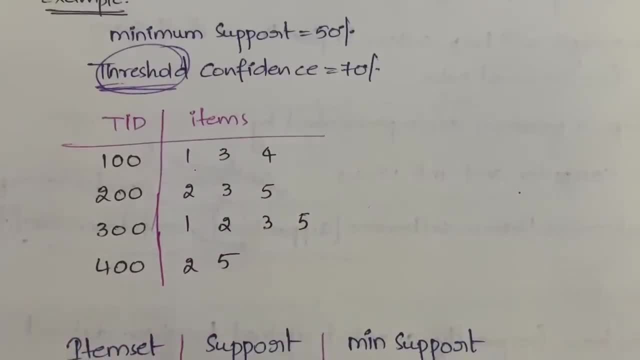 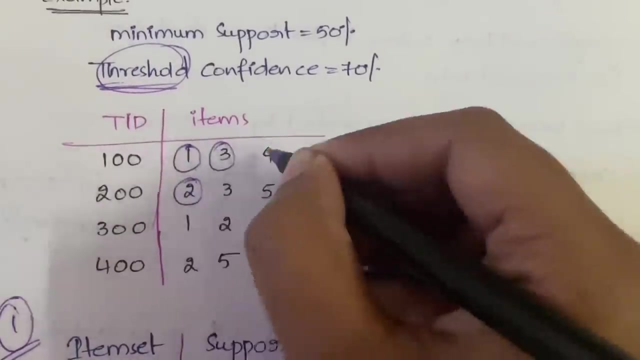 So this is our example. Okay, now we have to start applying our priori algorithm. In the first step, what you have to do is you need to write the frequency of each and every item. Okay, so that is here how many items. you have one distinct items: 1,, 2,, 3,, 4,, 5, right. 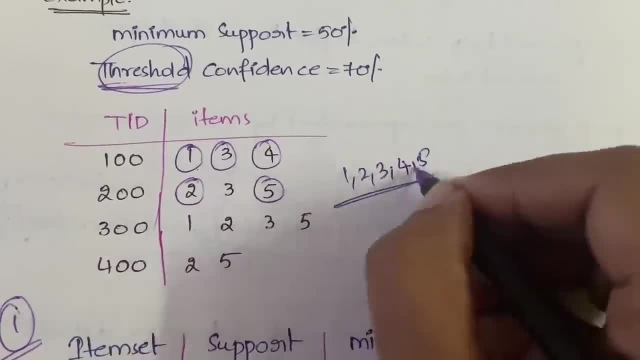 So we have 1,, 2,, 3,, 4, 5.. So for each, for 1,, for 2,, for 3,, for each of the data item. for the item set we have to write the frequency. 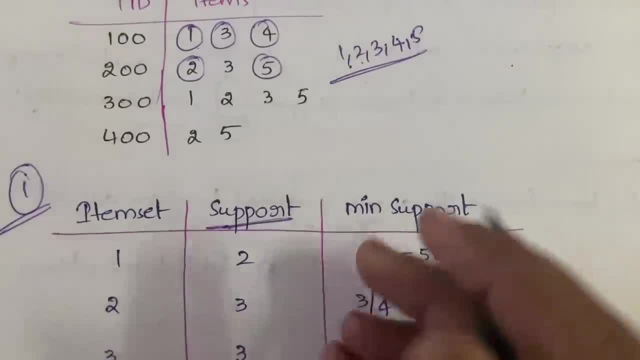 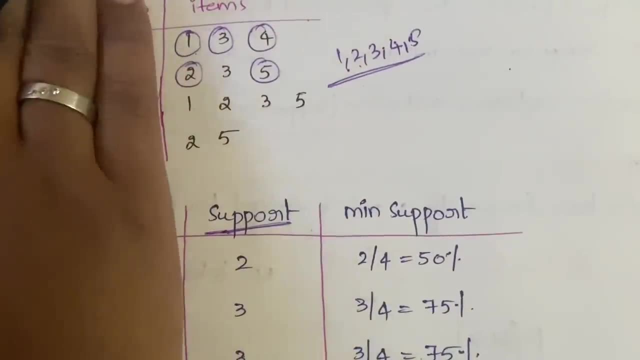 Okay, How. I will tell you That. frequency is nothing, but it is represented as support. First item set: 1.. How many times 1 is repeated in the all? Now, irrespective of transaction ID? you have to not think of transaction ID now. 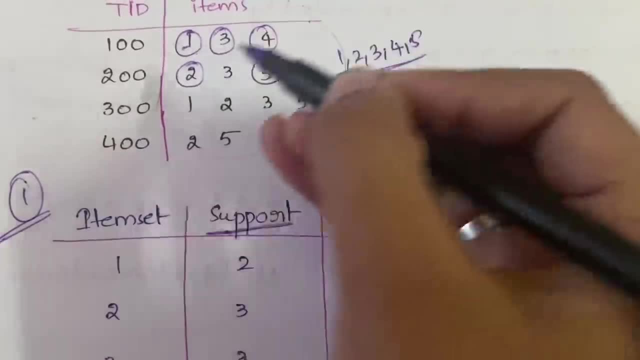 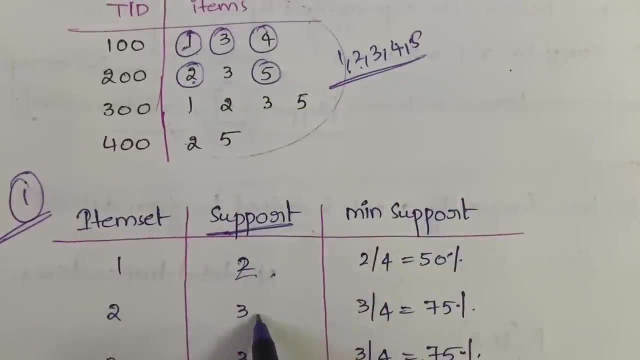 Okay. So 1,. how many times it has occurred? 1,, 2.. So the support of 1 is 2.. Okay, Next 2.. 1, 2, 3.. So the support of 2 is 3.. 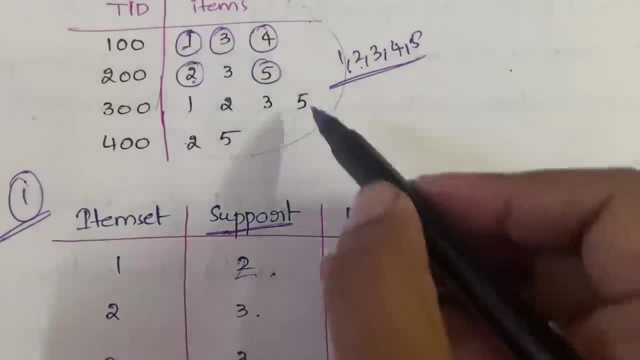 Okay, Next 3. 1,, 2. So support no no. 1,, 2,, 3, right, So the support of 3 is 3.. Next, 4. 4, only here. 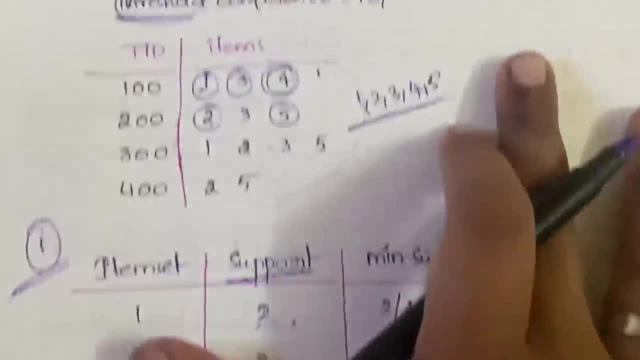 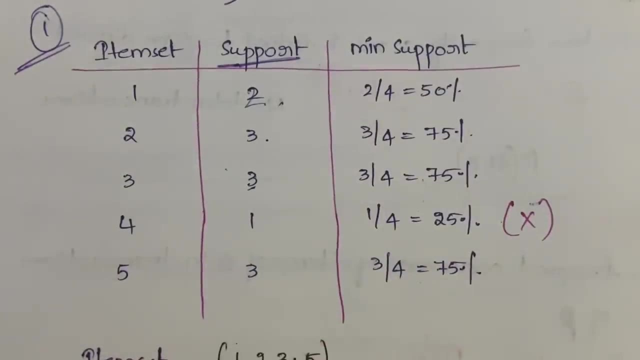 Only 1 time, Nothing, nowhere. So support of 4 is 1.. Next 5. 1,, 2,, 3.. So support of 5 is 3.. Okay, Now, after getting the support, you have to calculate the minimum support. 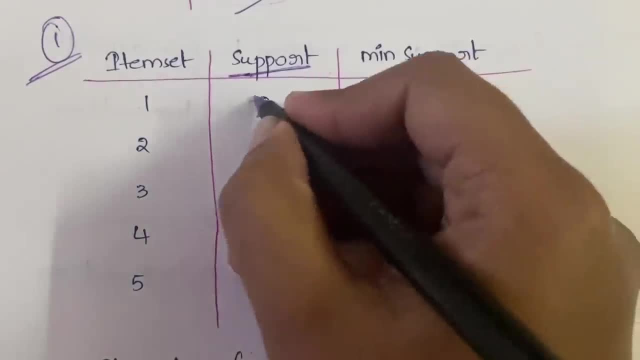 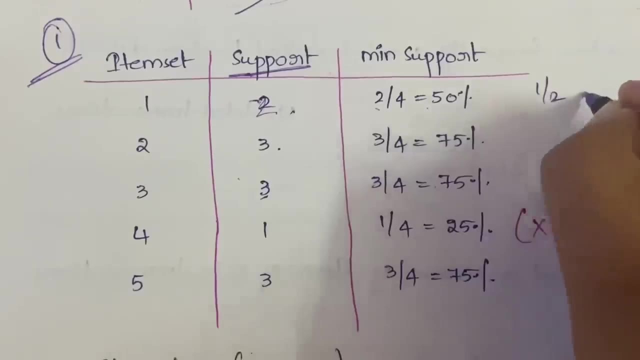 How you will calculate the minimum support, The support divided by total number of transactions. How many? you have? 4, right, So by 4.. Okay, 2 by 4, you will get 1 by 2, which is nothing but 50%. 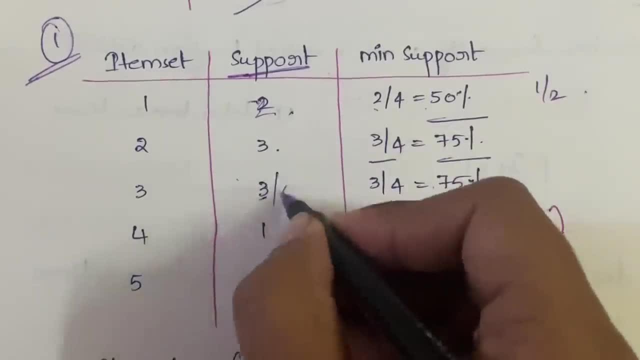 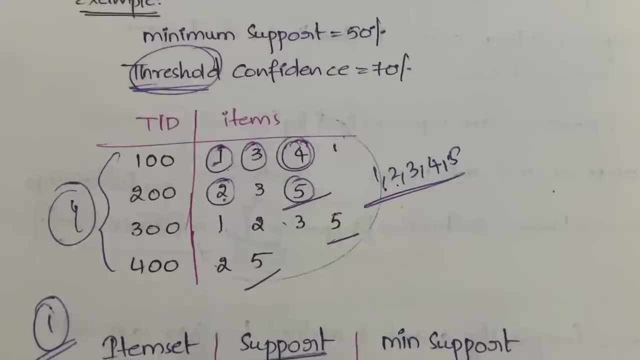 3 by 4 is nothing but 75%. Again, 3 by 4.. 1 by 4, 3 by 4. like that you will get the minimum support. after getting the minimum support, go back to the question again: what initially what we have defined as minimum support? 50 percent, right? so? 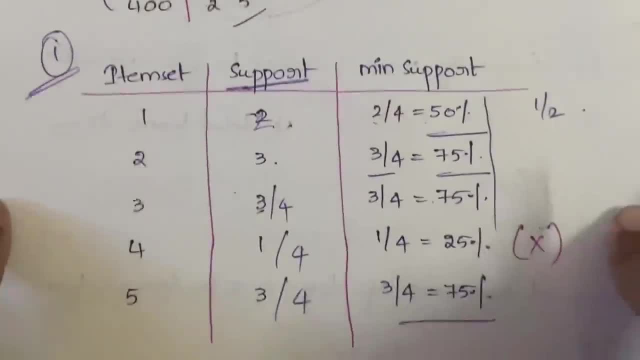 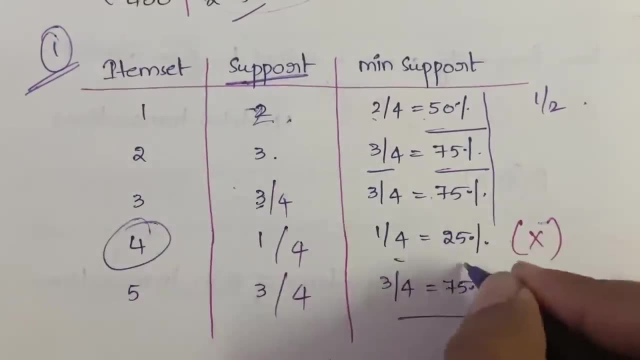 whatever are below 50 percent, you have to cross them. that is for the next iteration. you will not consider it so which is having below 50 percent? this 4 is having only 25 percent, right, so you can cross it, that is. it is eliminated. now what is the item set? new item set that you got. 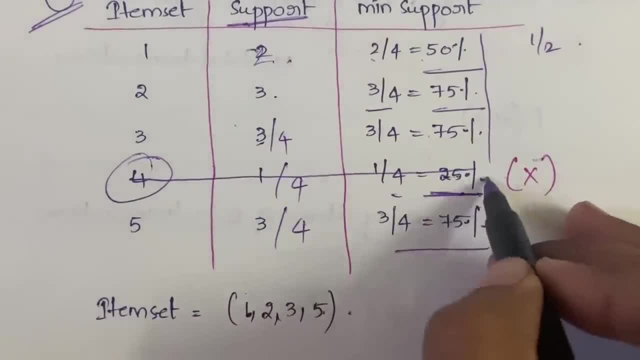 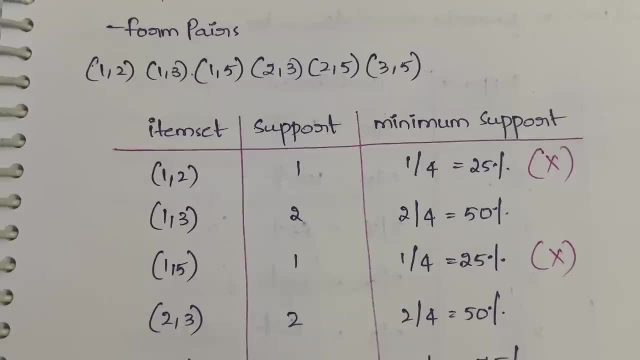 1, 2, 3, 5, no 4. okay, because it has less than 50 percent right. so 1, 2, 3, 5 is your new item set. now what you will do is with that- 1, 2, 3 and 5- you have to form the pairs. okay: 2, 2 pair in the sense. 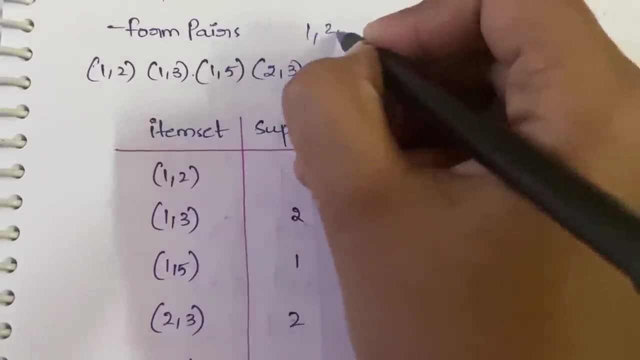 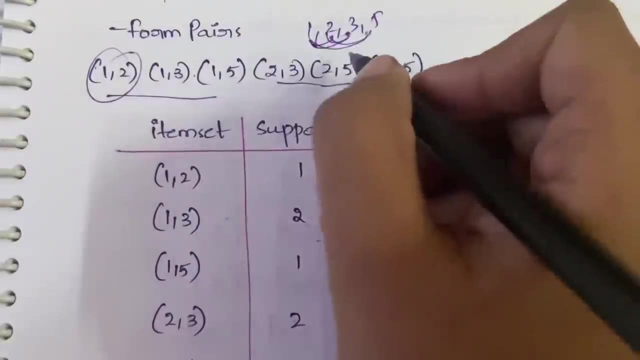 2 only. right, so 1, 2, 3, 5. right, so 1, 2, 1, 3, 1, 5. next 2, 3, 2, 5, 2, 1 is already formed. 2, 1 or 1, 2 represents. 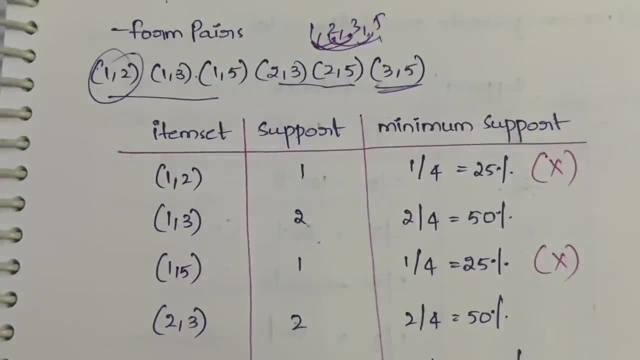 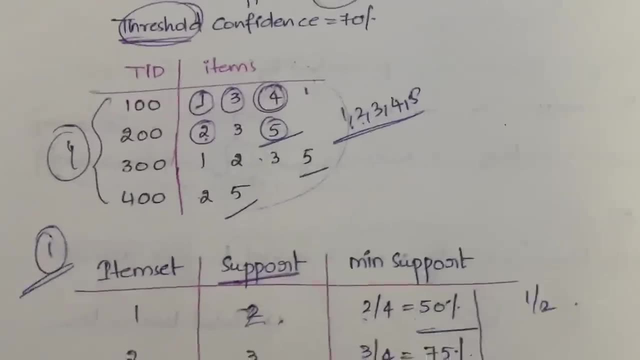 the same. next is 3, 5, so we have to form the ordered pairs. after you form the ordered pairs, now you have to write all these ordered pairs into an item set, like how we have done here, like we have written each and everything right in the same way here in the 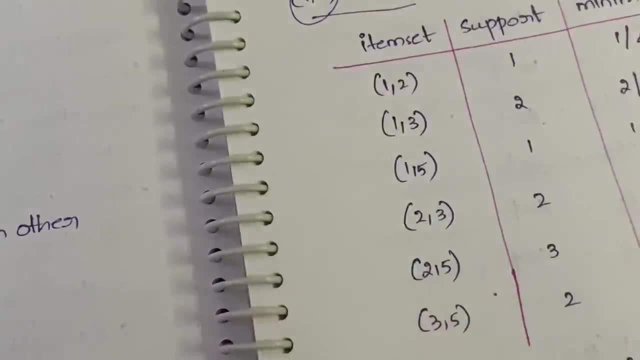 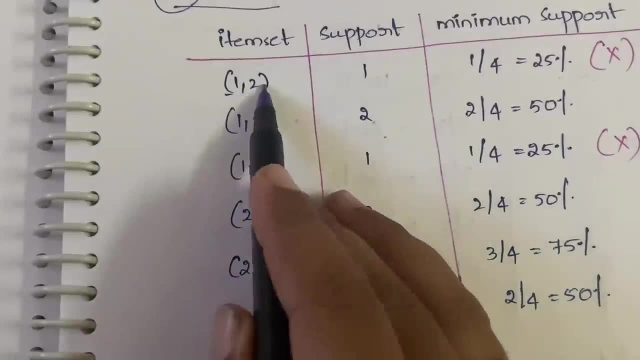 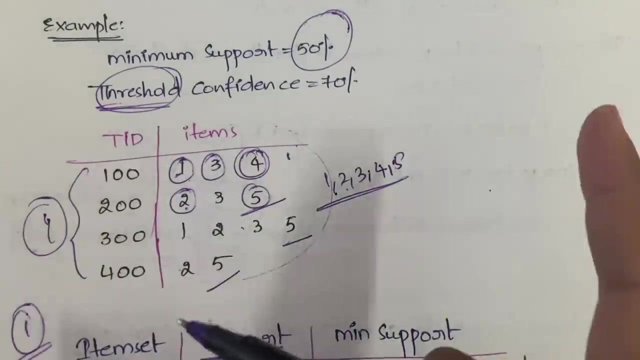 second step. what you have to do is you have to write the ordered pairs directly. got it. so once you write the ordered pairs, then you have to again calculate the frequency. so 1, 2, what is support of 1, 2? see 1, 2. support, how you calculate, is 1 and 2 together, where they have how many times they. 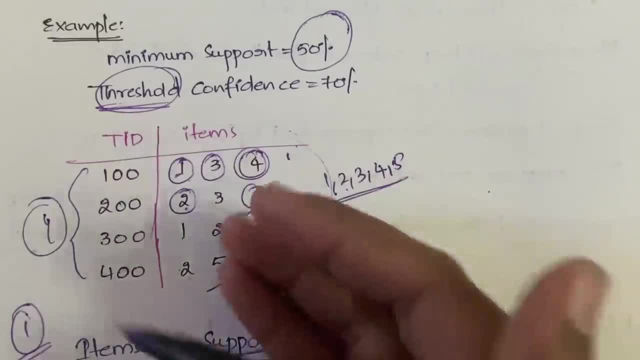 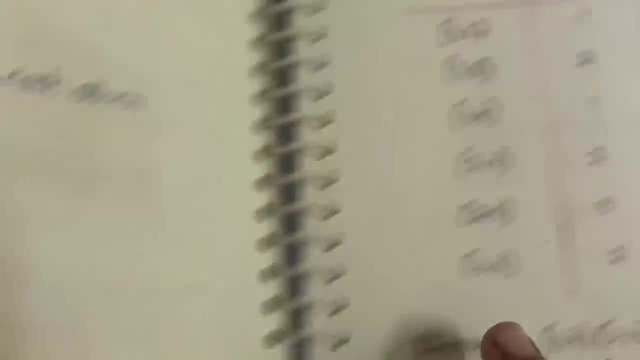 have occurred in single transaction. 1 and 2 together has to happen. how many times happened? only once: here no 2. here no 1, here also no 1. so only once it has happened, right, so the support will be 1, next 1, 3. how many times it has occurred? 1 and here in the third transaction, 2 times. so 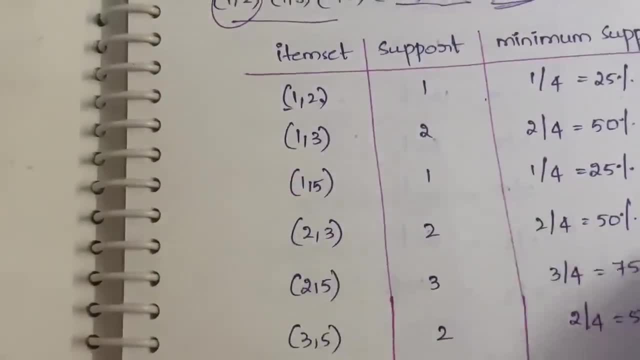 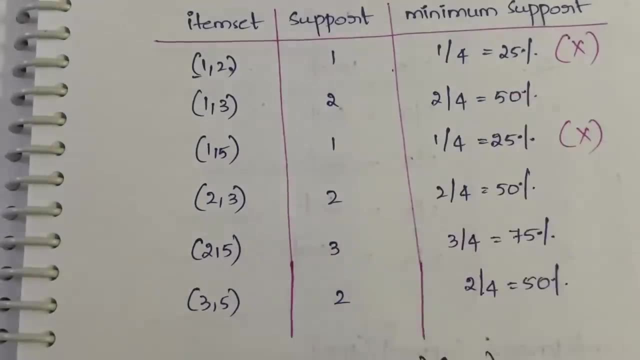 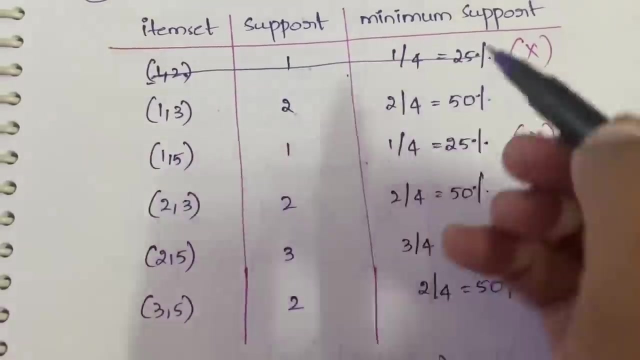 its support will be 2. like that, you have to fill the support of each and every ordered pair from the table. initial table got it, and then again you have to calculate the support dividing by 4, because total 4 transactions are there. so here also you got 25%, 25%. so these two things will be eliminated because our minimum support is. 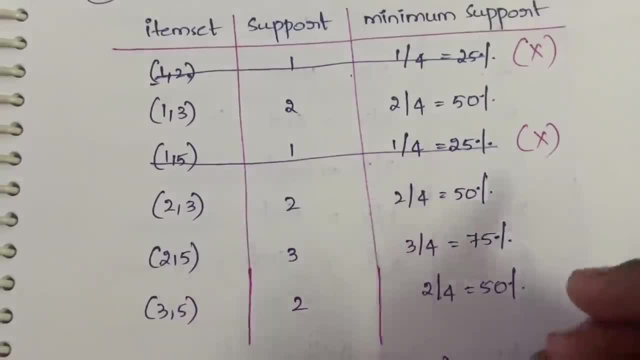 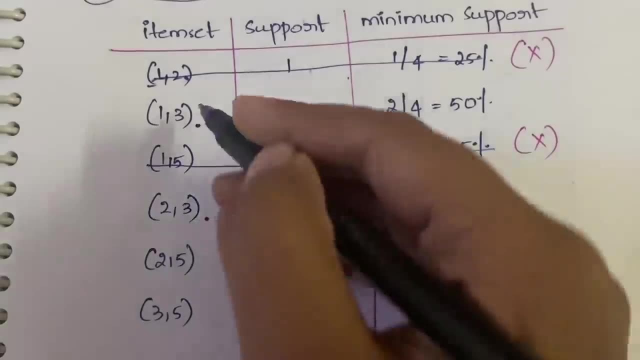 what? 50%. so it is less than 50%. we have to eliminate it. got it now. what are the ordered pairs? new item set that you will get: 1 comma 3. 2 comma 3. 2 comma 5. 3 comma 5. see, this is the new. 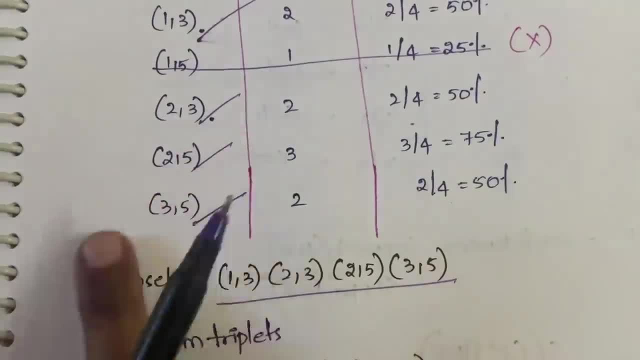 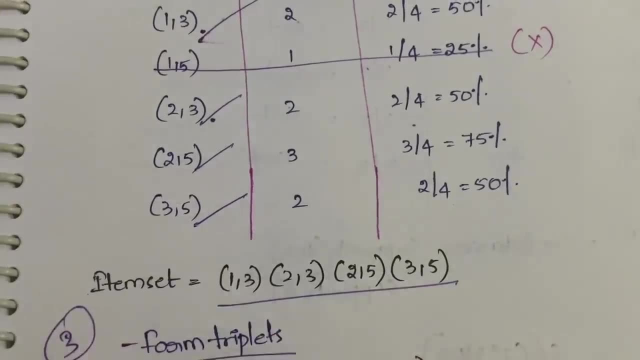 item set that you have got: 1, 3, 2, 3, 2, 5, 3, 5. new item set is generated now from this new item set in the third step. what you have to do is you have to form the triplets- see simple in the first step- like single values we have taken in the second. 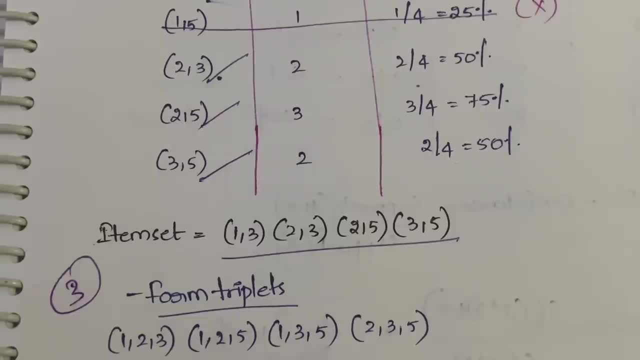 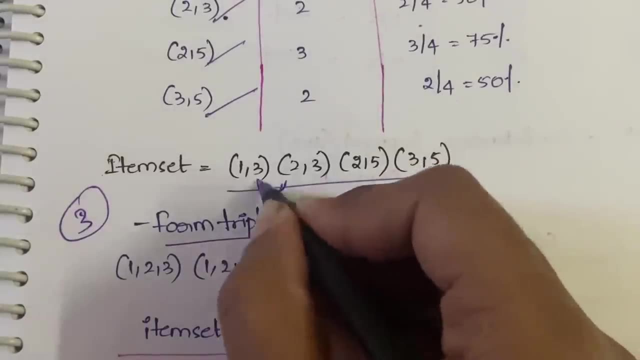 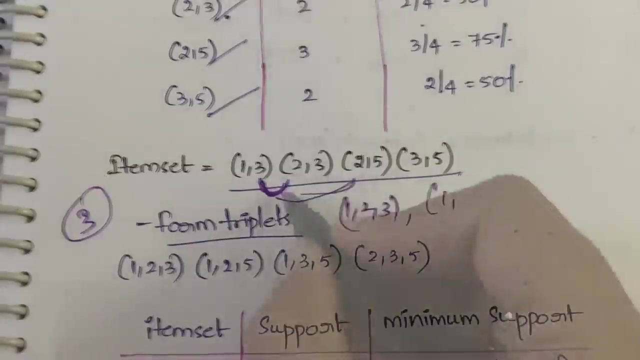 step we have formed ordered pairs like 2, 2 values. and when the third step, we are forming tripling triplets. that is, we are taking 3, 3 values. got it now let us form the triplets from these two things. what you can form: 1, 2, 3. next, from these two things you can form 1. sorry, you cannot form. 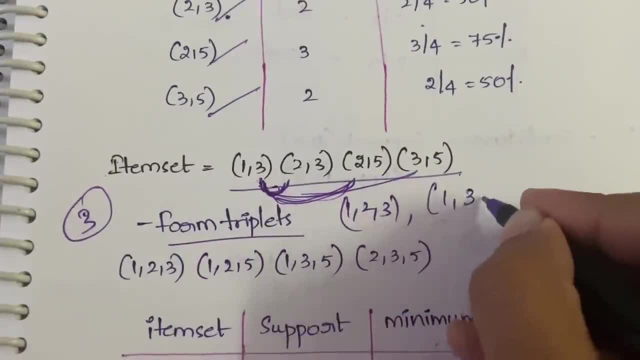 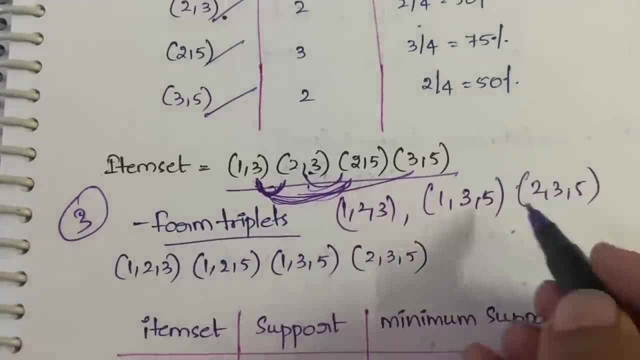 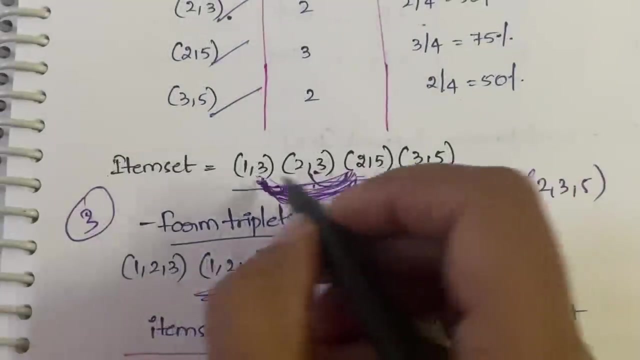 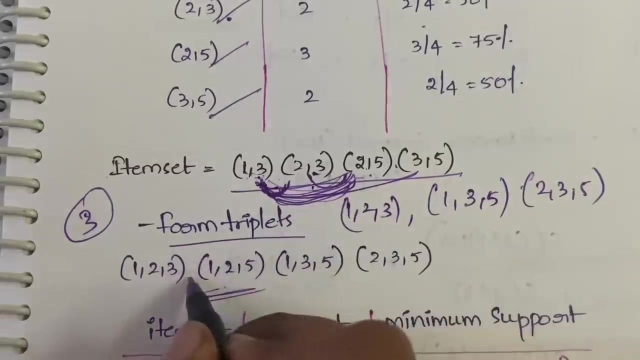 anything, because nothing is common from these two things you can common, you can form 1, 3, 5. from these two things, only 1, 3, 1, 2, 3. you have already formed. so 1 3, 5, we can form. so 1 3, 5 and next. yeah, so like: 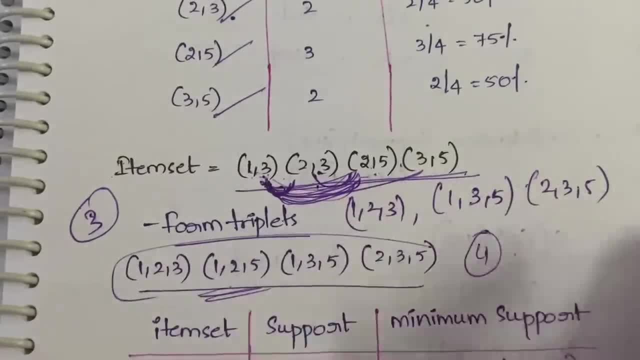 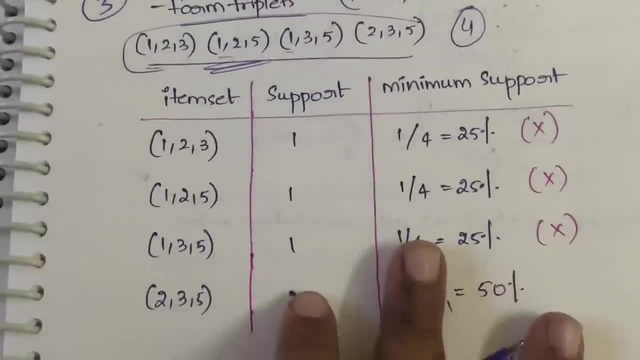 that all the triplets will be formed. you get 4 triplets out of these. you know combinations, okay, once you get the triplets, now the same process for these triplets: you have to calculate the support. we have taken all these four here and now we have to calculate support. how do you calculate support? 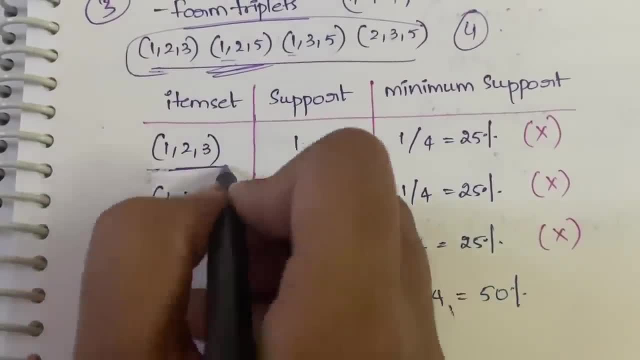 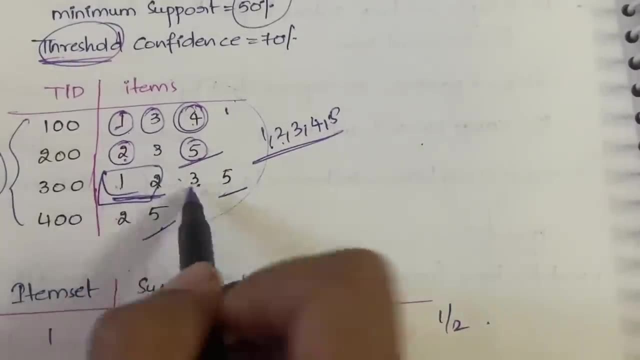 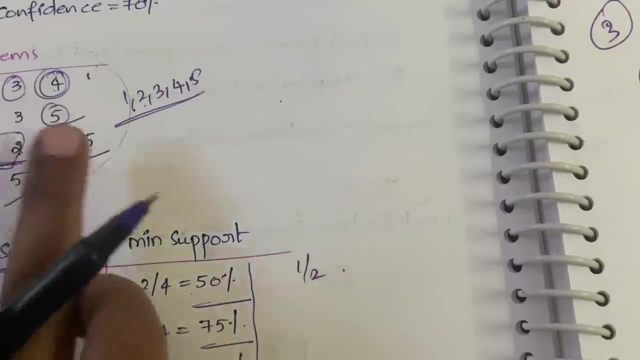 then one, two, three. how many times it is occurring in a complete all? one, two, three, three has to come in a single transaction. that is happening for how many times? let us see one, two, three one time. so the support of one, two, three will be one next to one, two, five. one, two, five. see one, two, five again. 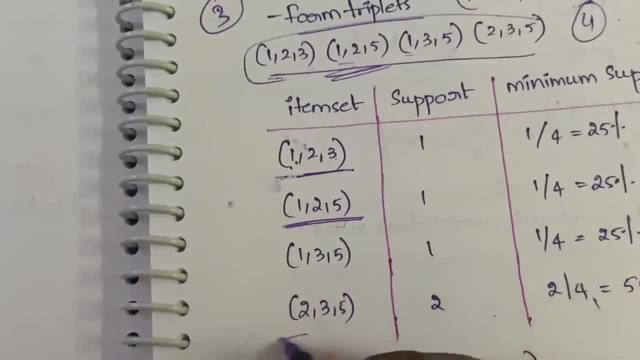 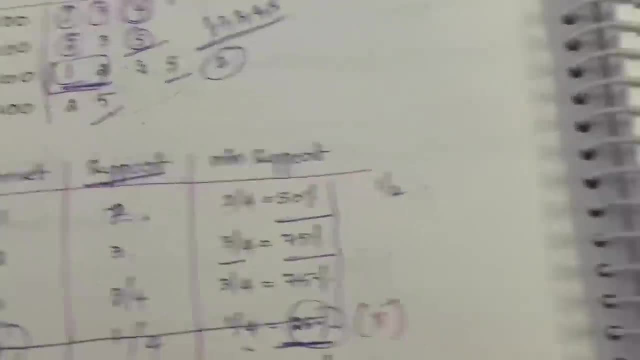 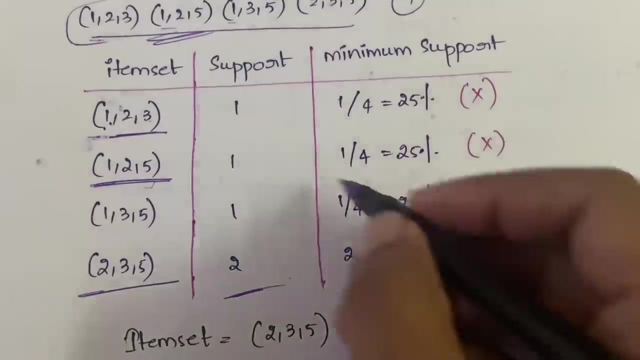 one time, right like that. you have to fill the tables for two, three, five, see two, three, five. two, three, five. how many times? two times, right? so since it has happened for two times, it will have the support as two and you have to calculate the minimum support by four. then you will be getting. 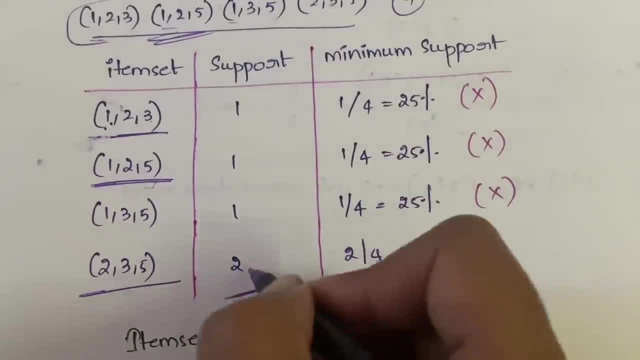 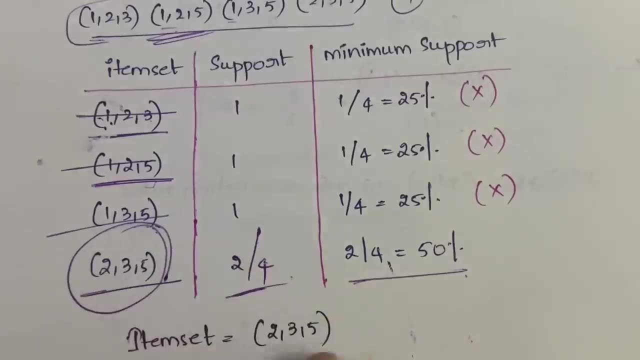 all 25s only, right. so only this one. you got it as 50 because 2 by 4, right? so now these three things will be eliminated. so the only item set that you have obtained at the end is 2 comma 3 comma 5. 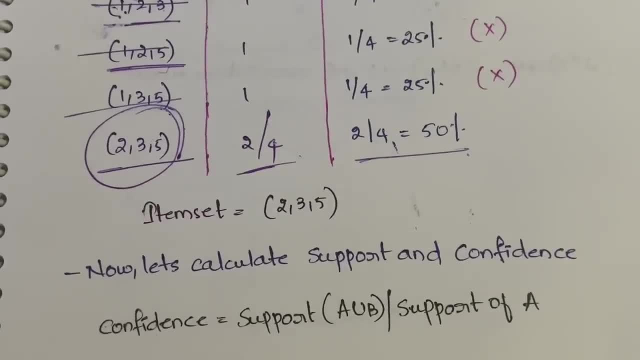 okay, now, for now, you have to calculate the support, and confidence got it. so how do you calculate the support? how do you calculate the confidence? i'll tell you, and for confidence, the formula is: confidence is equal to support of a union b by support of a. so what is support of a union b? what? 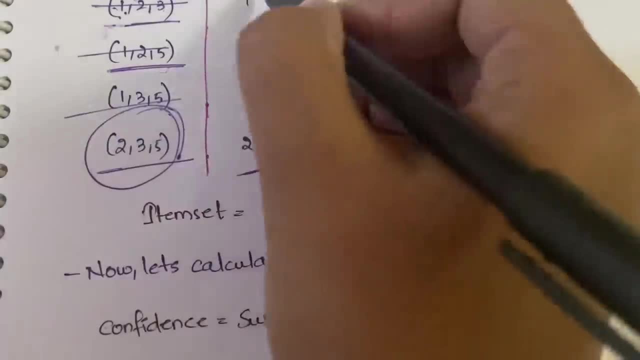 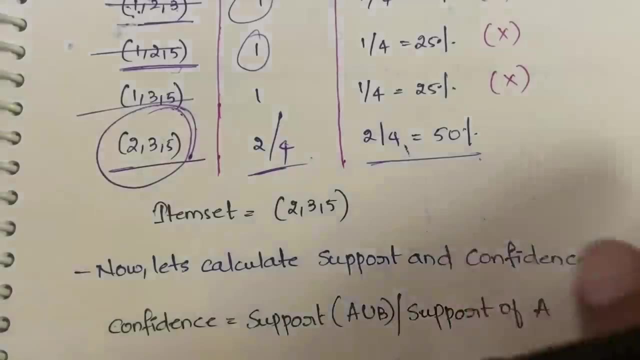 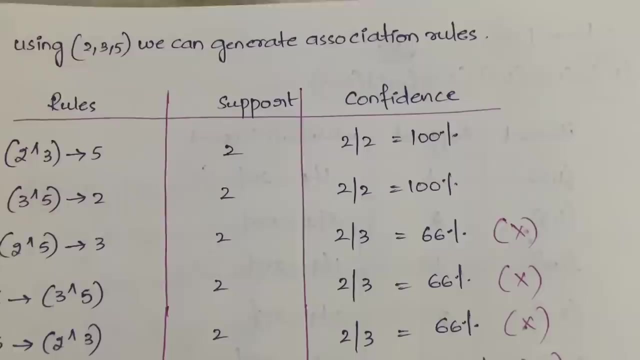 is a, what is b? everything i'll tell you. don't worry, support is nothing but discount. you are clear about support right now. how do you calculate support of a union b? i'll tell you first. before that, we have to write the association rules. okay, so so, using two, three, five, you have to generate the association rules first. generating association. 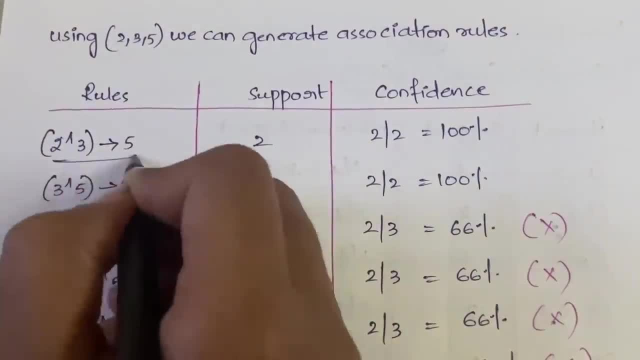 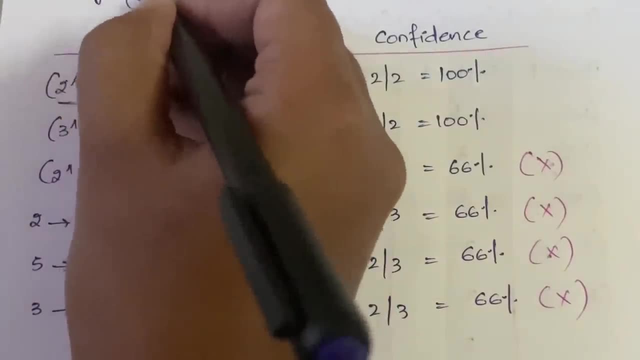 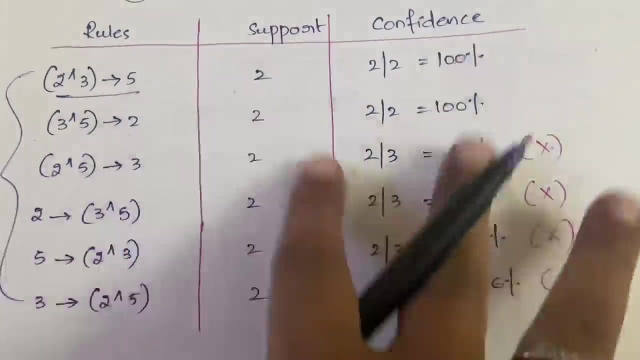 rules is very simple. see two, three, five, three, five, two, two, five, three, now individually, like two, three and five, three, two and five, five, two and three. like that. you have to generate. you'll get six association rules, got it. so once you generate these six association rules, you have to calculate. 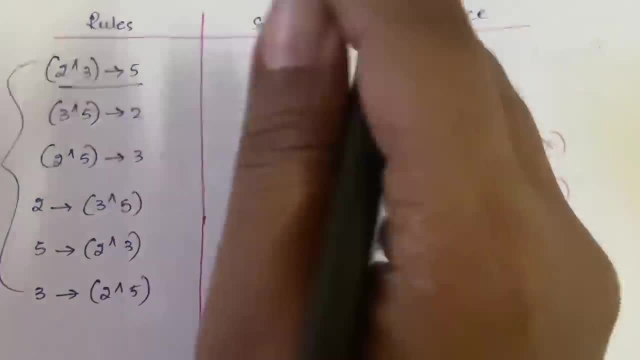 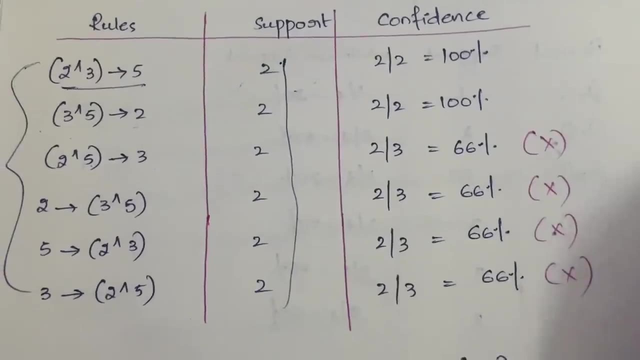 the support and confidence. support is always two, obviously two, because two, three, five commonly, how has occurred in our example? for two times right. so the support is two for all. got it. now you have to calculate the confidence, which is very important. so first for this, i will tell you, for this rule i 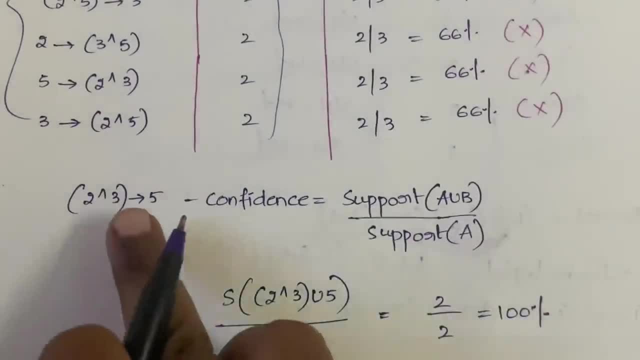 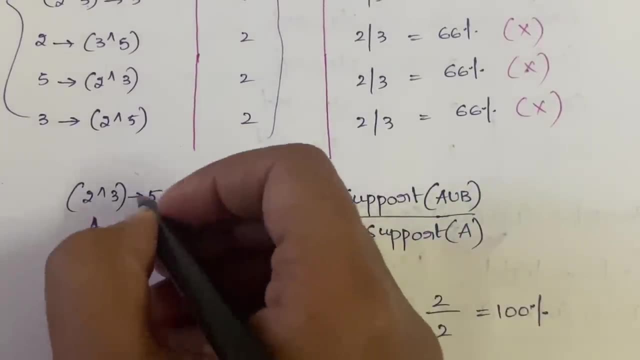 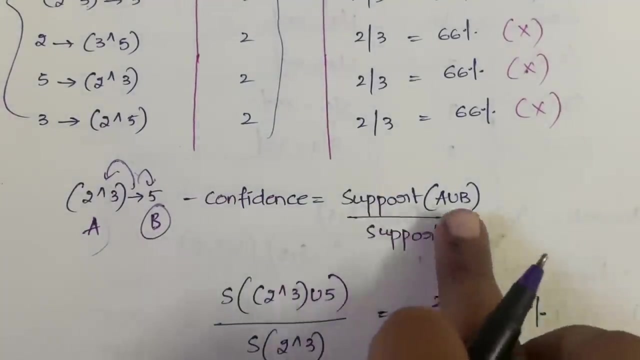 will tell you the confidence how to calculate. first, confidence is equal to support of a union b by support of a right. this is a, this is b, or the arrow mark which is on left side of the arrow mark. that complete term will be a right side of the arrow mark, it will be b. okay, support of a union b. 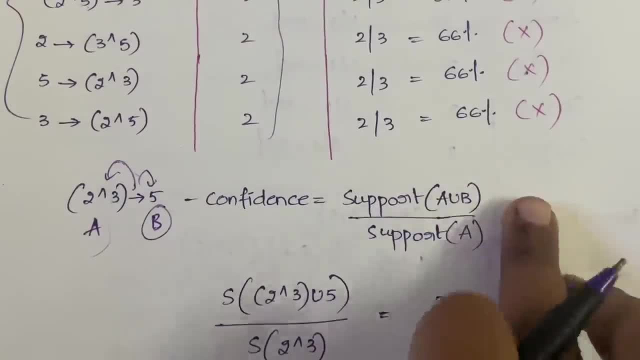 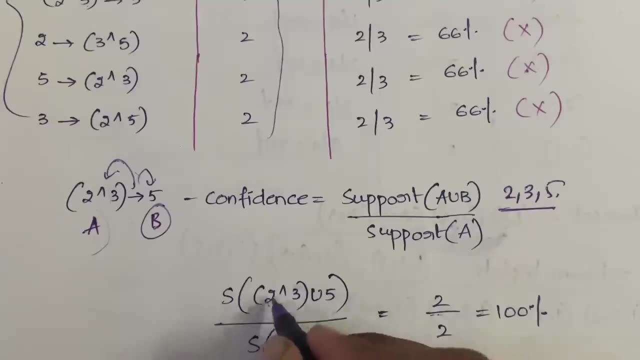 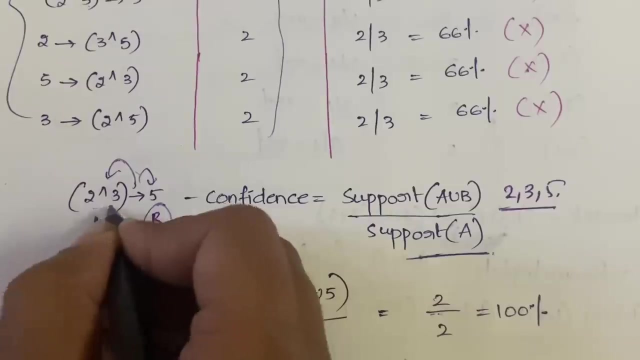 what is support of a union b? support of a union b is nothing but support of two, three, five, got it? what is support of two, three, five? it's two, right, see two cap, uh. two, yeah, two. and three. union five- yeah, see two by. and support of a support of a means only two comma three, right? so you have to find out. 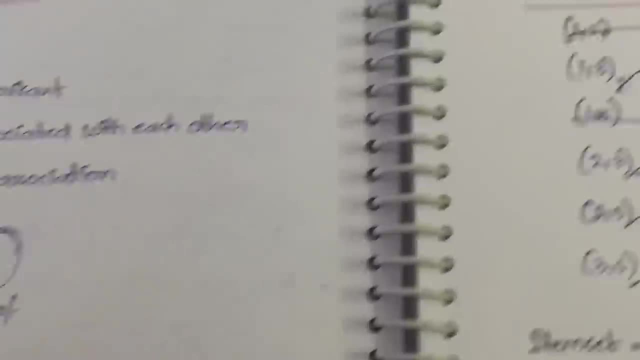 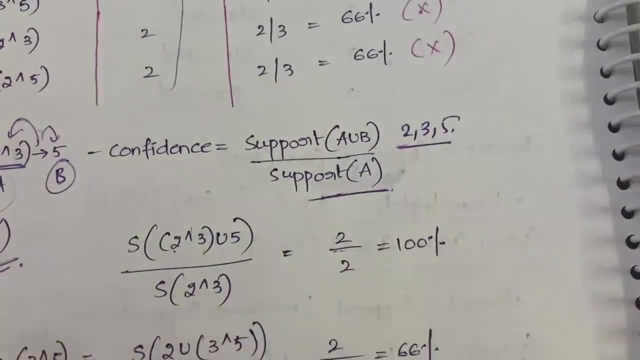 what is support of two comma three? i guess we already got it here in the previous. yeah, see, support of two comma three is two, like that. you have to see the previous tables and calculate the of a or support of a union b. okay, so support of 2 and 3 is 2. so 2 by 2 you get 100%. so here you. 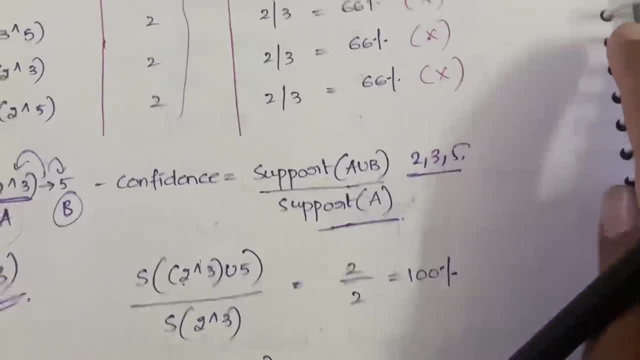 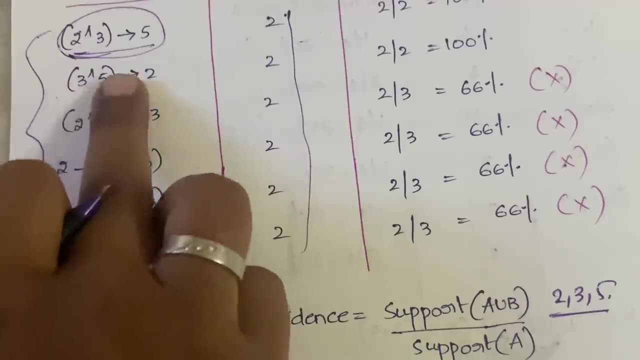 will be filling it as 100%. got it next like that. only you have to calculate for 3 comma, 3, 5, 2 and 2 5, 3. so here what a? what is a 3, 5, 2? obviously the above will be 2 only because if the, even though 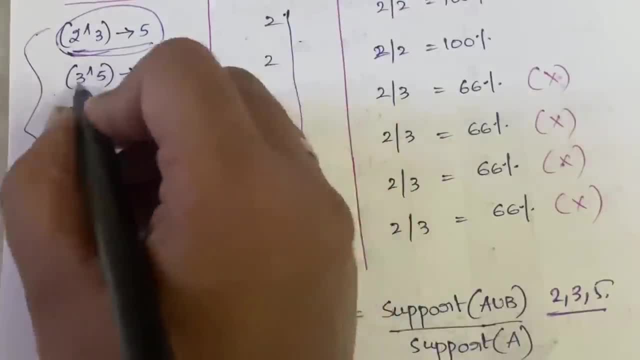 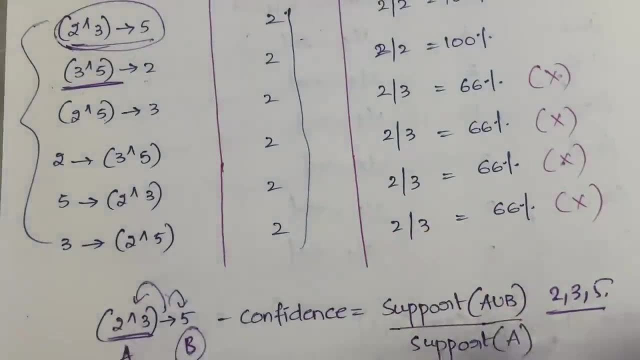 the order is changed. also, it is same rate: 2, 3, 5 only. but here bottom you have to calculate the support of 3 comma 5, so that you have to replace: okay, like that. and another example also have done like this: this three are different. right, these three are one set and these three are one set. 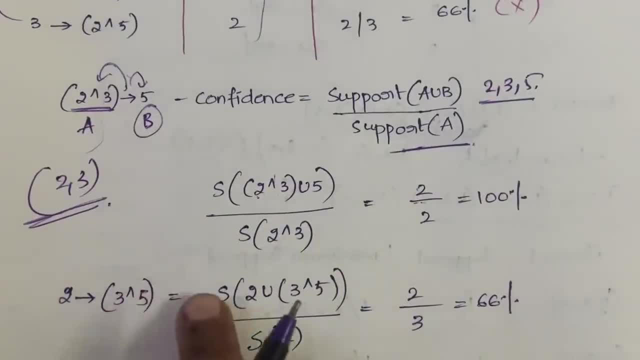 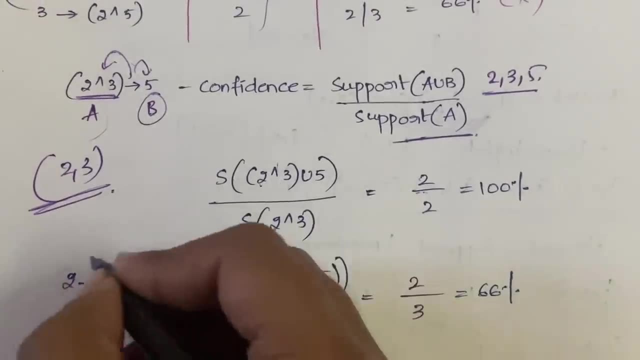 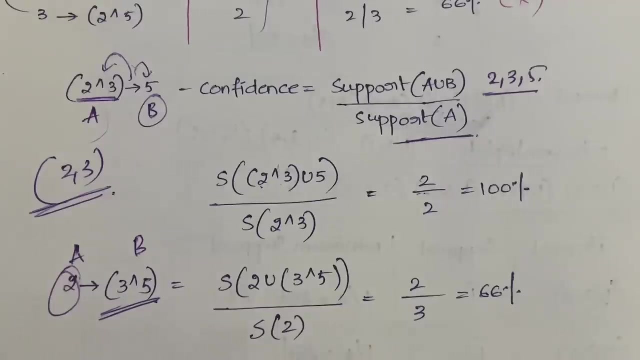 for these three. how to calculate? is 2, 3, 5. so support of 2, union 3 and 5 by support of 2. you have to take y 2 because see here a is only a, only two, b is three and five got it. so support of only two. what is support of two? here it is three. 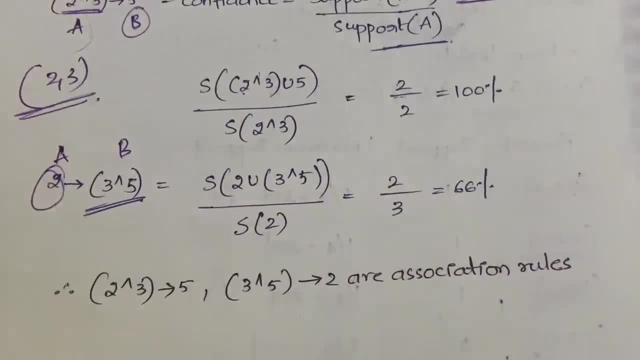 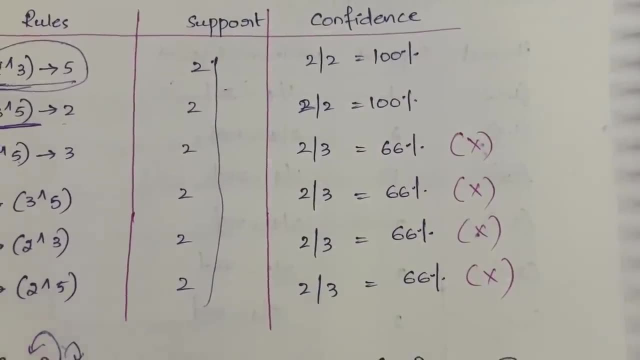 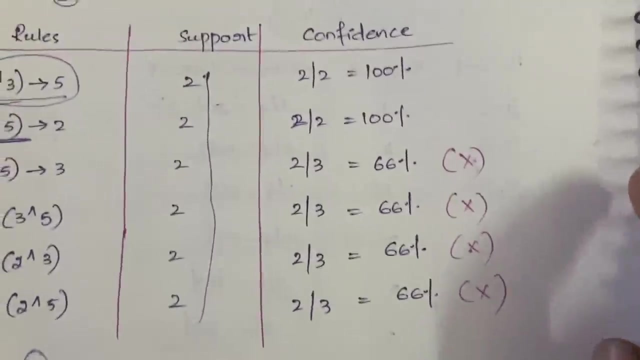 right. so two by three, that is 66 percent. okay, now, once you calculated the confidence of all the values, now what you have to do is you have to you what is the threshold confidence that you have taken? 70 percent. so whatever are below 70 percent, you can cross them, that is, you can eliminate them. 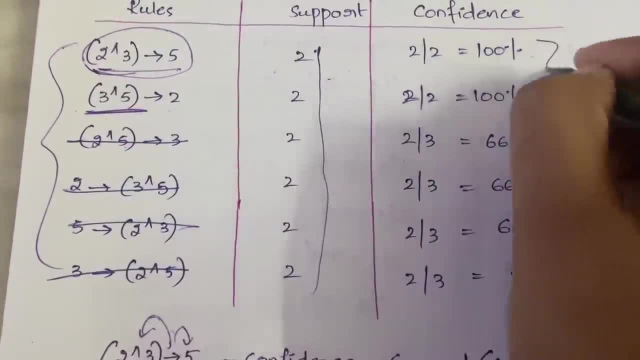 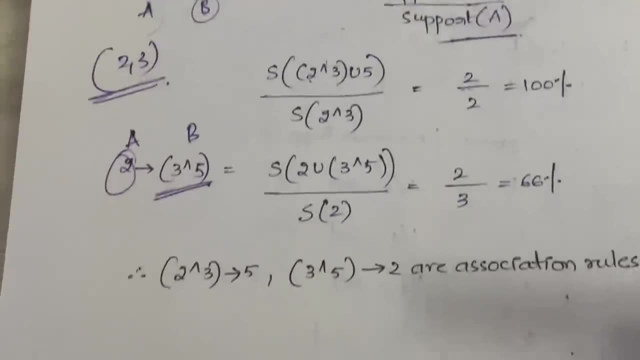 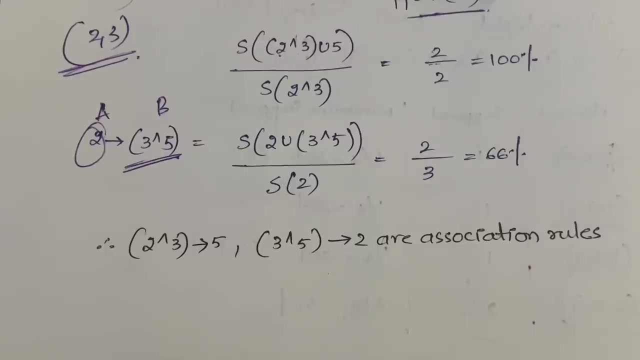 so you can eliminate this, this, this and this. only these two association rules only have to be considered. among all the association rules generated, only these two are the strong and the perfect association rules which will give you the relationship between the objects. got it? this is a priori algorithm. i tried my level best to make it very clear to you, but still, if i was not able,